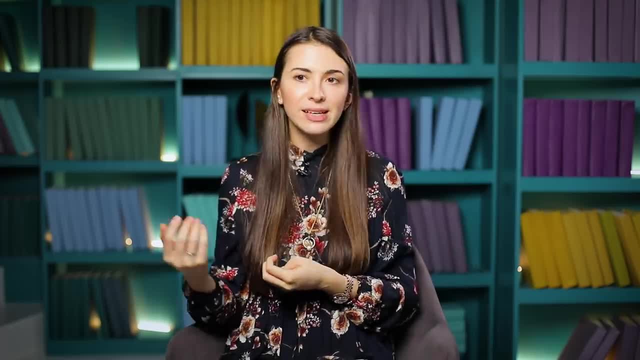 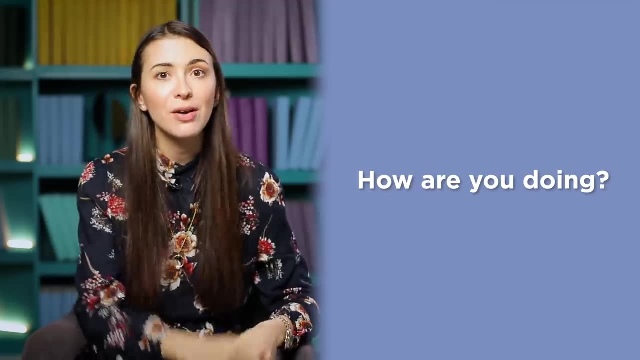 phrases in English written down. learn some of them At least, like: how are you doing? You know, instead of thinking: oh, what should I say? How are you Or how is your day going? Whatever You learn one- How are you doing, And you know what this phrase means. Learn all of those intro phrases. 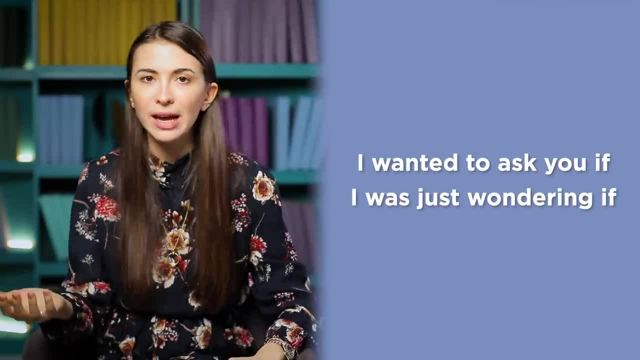 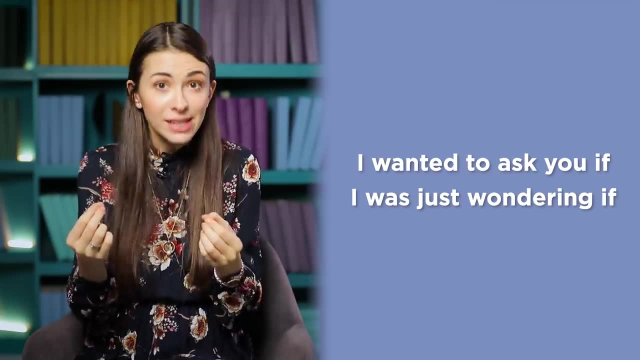 I wanted to ask you if I was just wondering if You know all of those phrases. again, they take away the pain of thinking how should I phrase this, And once you're pronouncing this phrase, you can actually think about the content that comes. 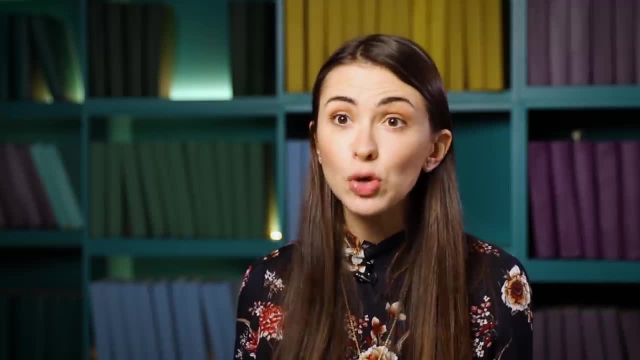 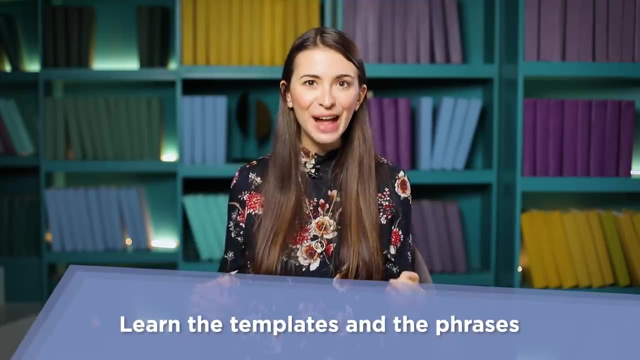 later, And this advice also works for exams. So, for example, if you're taking TOEFL or IELTS and if you're afraid of the speaking part, learn the templates. learn the phrases. They're going to help you sound smoother, And the same with conversational English: Learn the phrases. 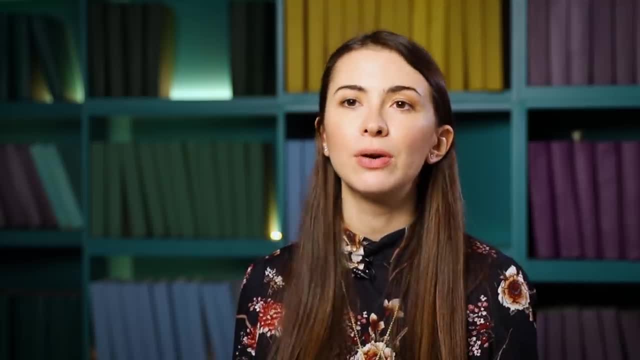 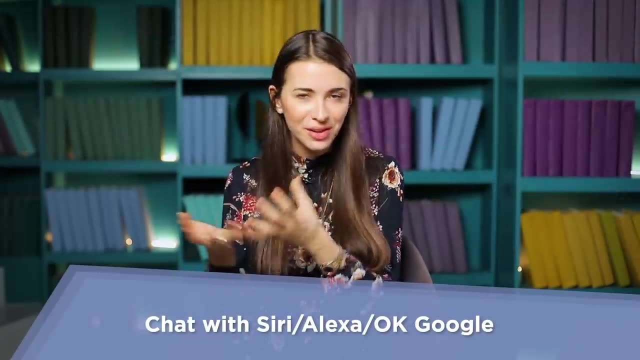 learn the structure, write down all the phrases into your phone, have them in notes and use them when you speak. The next tip is to chat with either Siri or Amazon Alexa, or whatever you have on Google- Okay, Google. I've noticed that so many times when some of my Russian friends started. 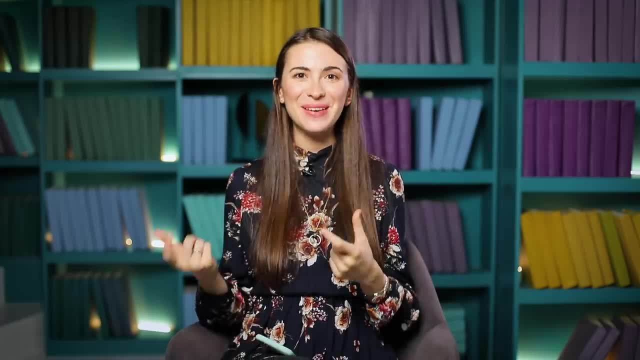 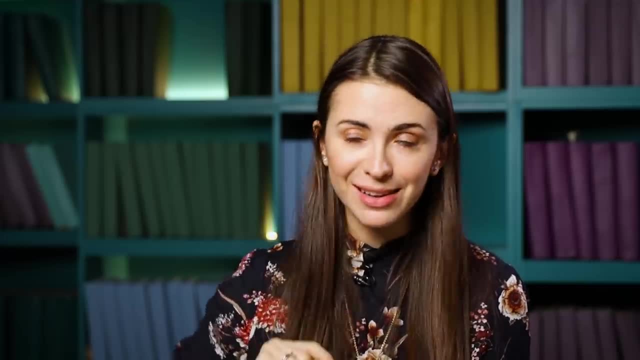 talking to Siri, she would not understand what they meant because of their pronunciation. And this is a very good practice, because if Siri does not understand you, something is wrong with your pronunciation. Yes, sometimes they have bugs and sometimes you just pronounce the word in a. 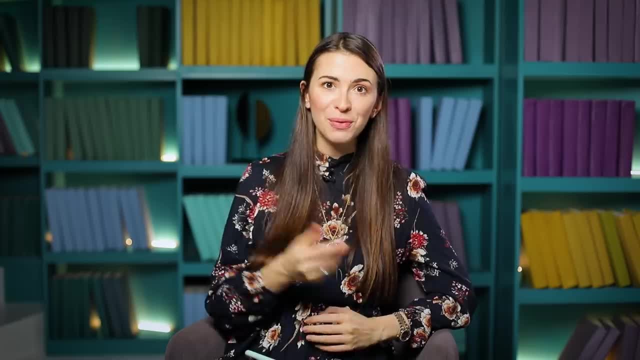 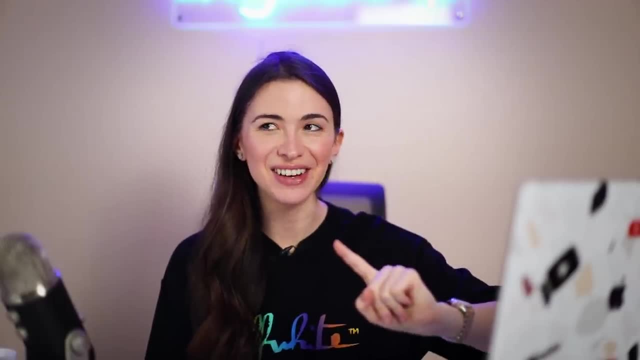 different way, But the thing is it is really helpful. It's really helpful. It's really helpful because you're getting instant feedback. If Siri didn't get you, then something was wrong. Quick pause here, guys. I know a lot of you are like, but Marina. 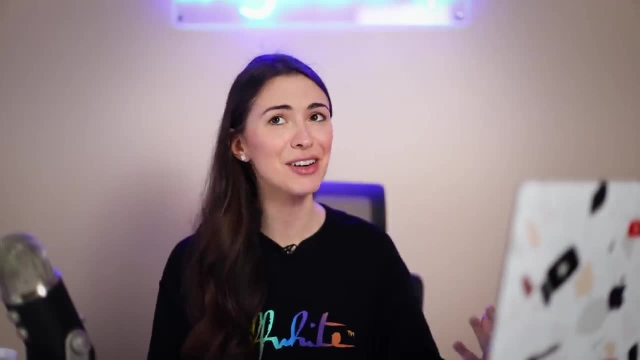 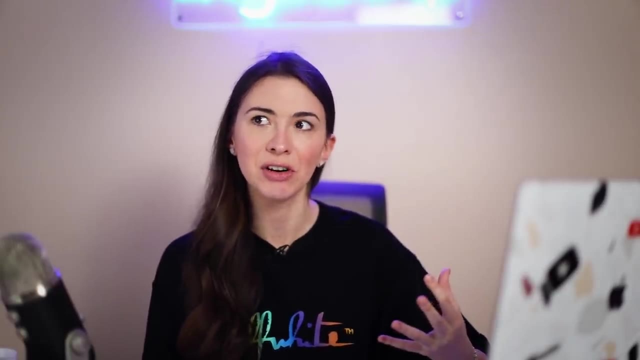 how do I work on my pronunciation? Yes, learning words is amazing, Learning phrases is amazing. But what if I speak and native speakers don't understand me? And it is really expensive to hire a native speaker to correct your pronunciation. Luckily, we are in the 21st century where 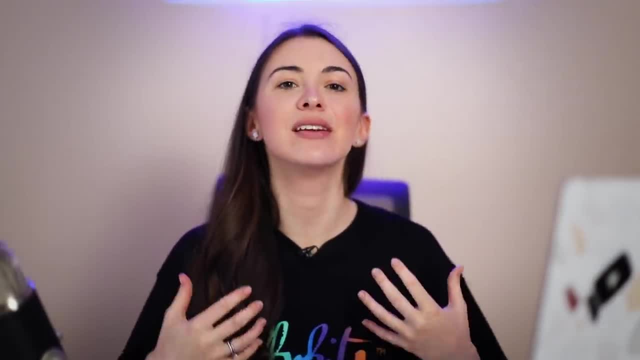 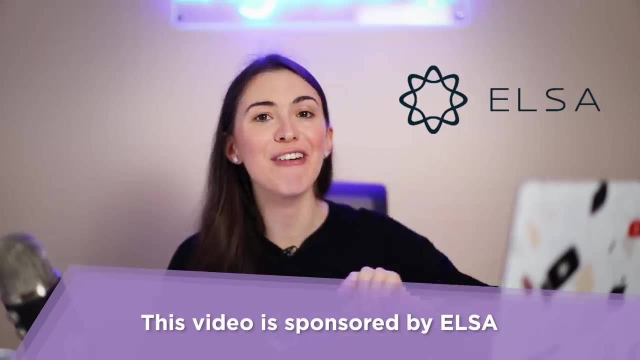 technology has gone so far that you can just download an app that is going to evaluate your pronunciation in English. The app is called Elsa Speak and it uses artificial intelligence to evaluate each and every sound that you pronounce, and it compares you to a native speaker When you 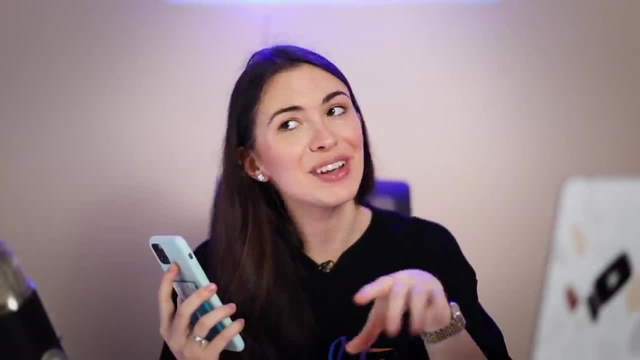 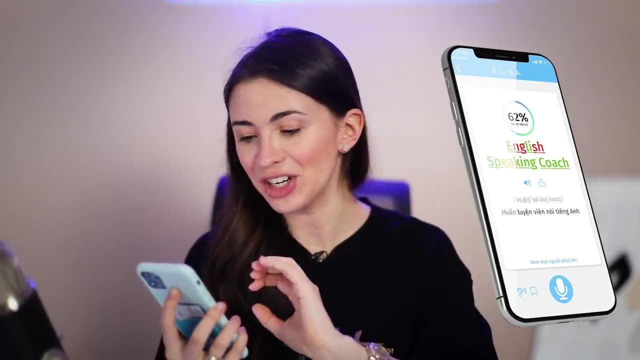 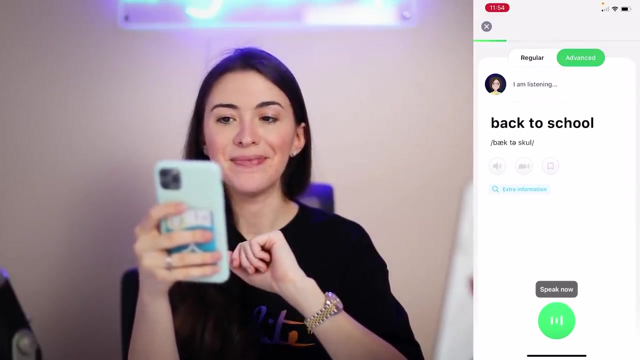 install this app. it's going to ask you what's your native language, because every language has its own peculiarities when you speak English. So I said everything to Russian and let's try. Let's see what it says. Okay, back to school. Let me pronounce it: Back to school. 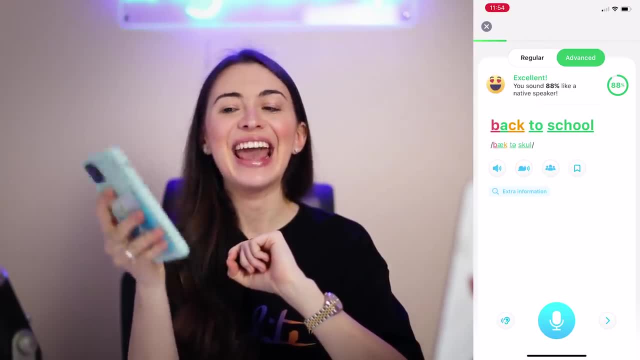 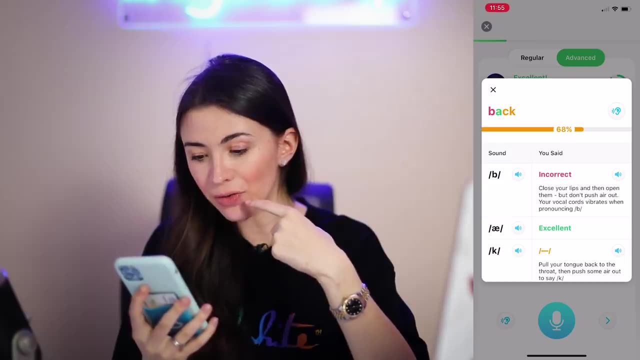 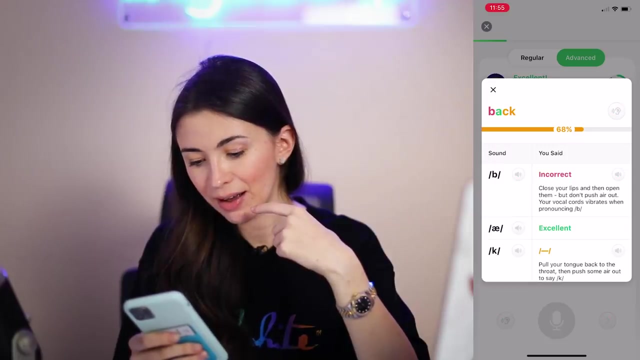 88%, like a native speaker. And now it gives evaluation to every single sound. So back, I think I was wrong with my B. Back Back to school. Close your lips and then open them, but don't push your out. 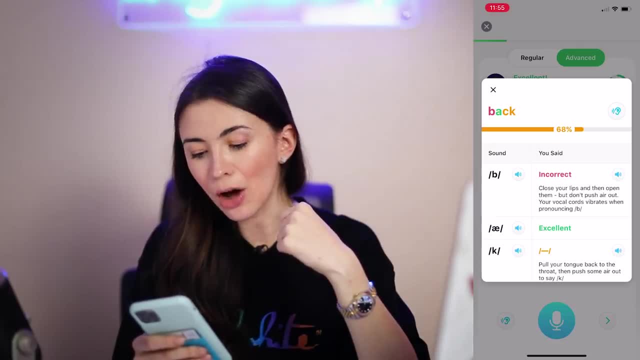 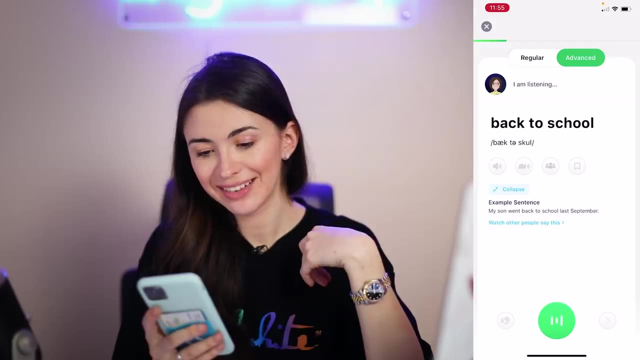 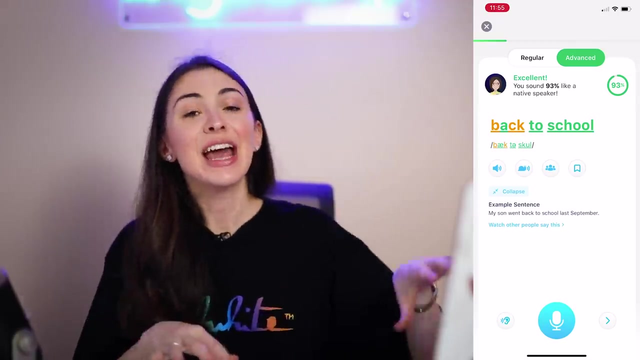 Your vocal cords vibrates when pronouncing B. Back to school. Okay, let's try again. Back to school, Yay, 93%. So this is the way it works. It evaluates every single sound And, apart from mastering your pronunciation, you will also enhance your vocabulary. 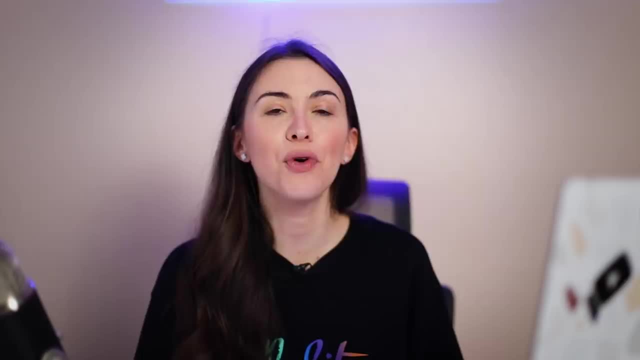 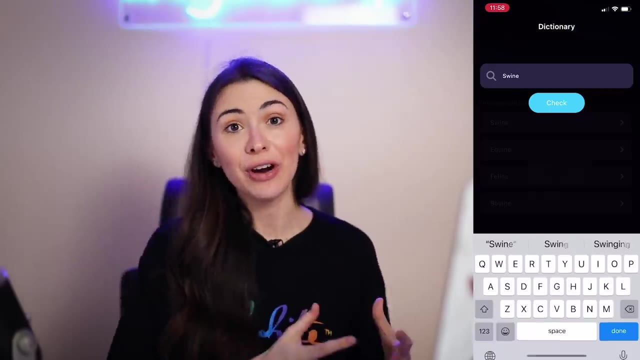 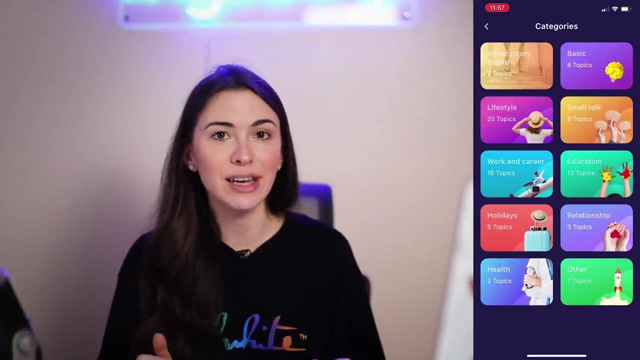 They have 1,600 plus classes on 400 plus different topics for you to go through. Elsa app also has a dictionary that helps you learn and learn to pronounce new words. I believe that Elsa Speak is one of the best apps out there to master your pronunciation. 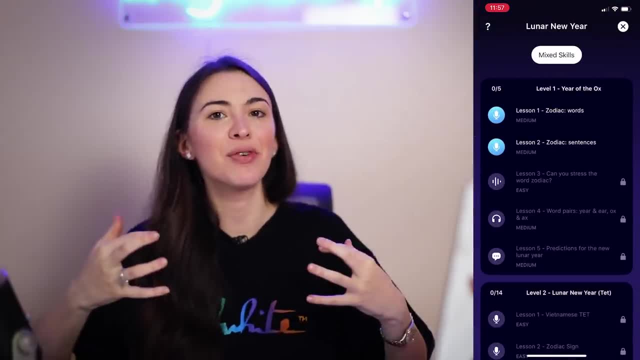 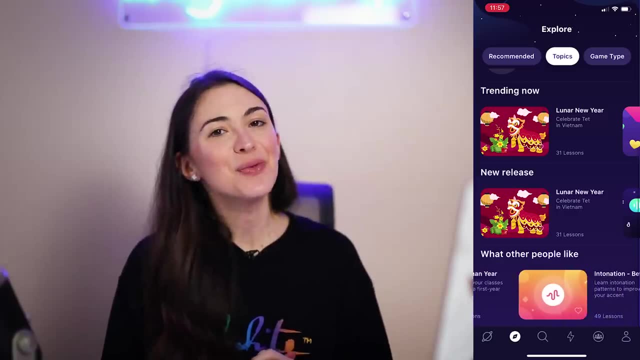 And to enhance your learning experience, because when you're learning from my videos, you're mostly like listening and writing down, but this is your opportunity to speak and get feedback And because you are watching this video, you're getting some special discounts. You can either get 85% on your lifetime subscription- so instead of paying almost $500, you get this discount and your lifetime subscription would be $94.99 cents- Or you can get a 30% discount on the annual membership. that will cost you $30,949., But you get a 50% discount. if you do not get this discount, so your lifetime subscription is $2.99.. So if you do get this discount, you get a 50% discount on your lifetime subscription and you get a $84.99.. So you can do that with education. 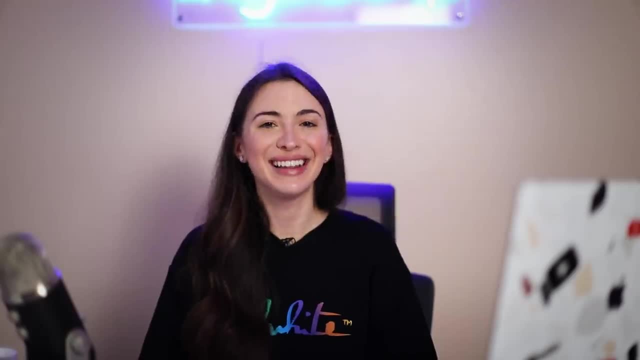 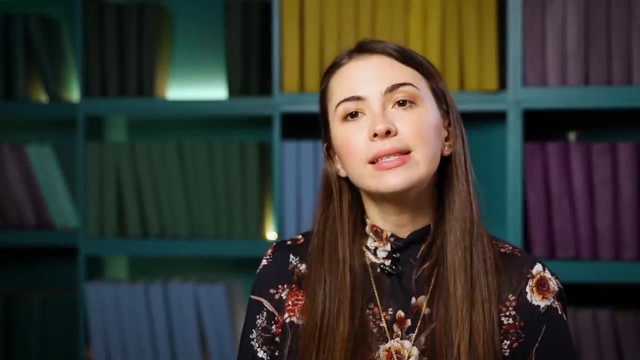 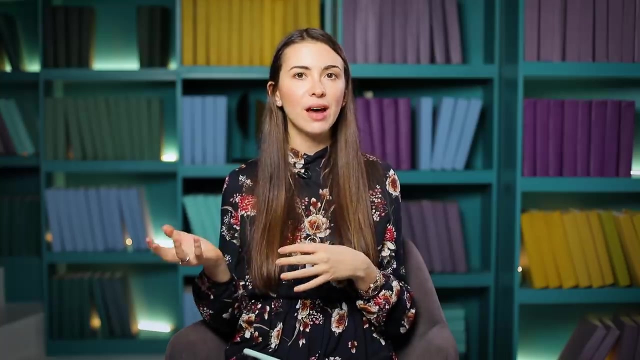 cost you 31.49. if you use links below this video, check them out in the description. and now let's get back to the class, the next tip that i use a lot. i used to use a lot. i no longer use it because i think i've mastered this, but anyways, when i was not living in the us, i would talk to myself every. 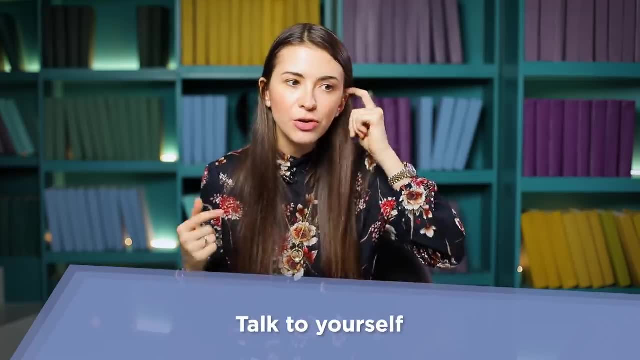 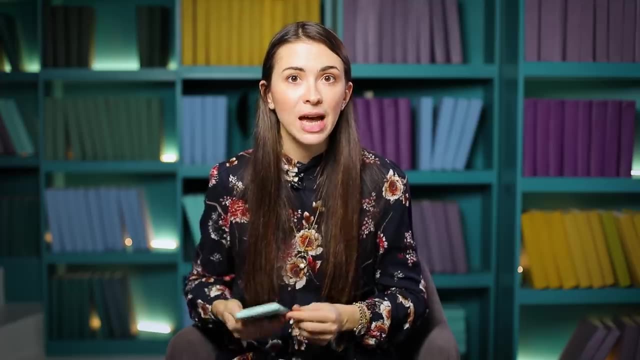 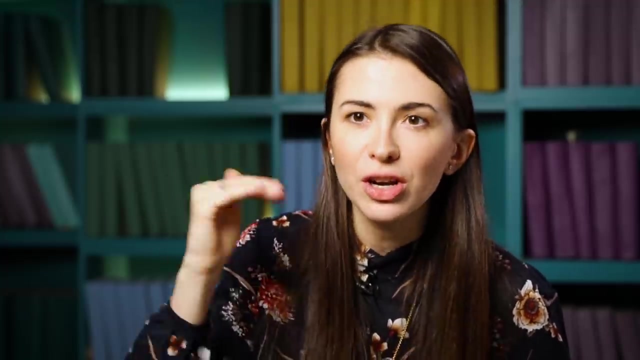 single day and whenever you're doing something in your head, just say it. i am recording this video for my channel. oh, i just got a message from my friend, i'm about to call my mom, i'm about to go to bed, and whatever you can do in english, just do it in english. just talk to yourself in your head. 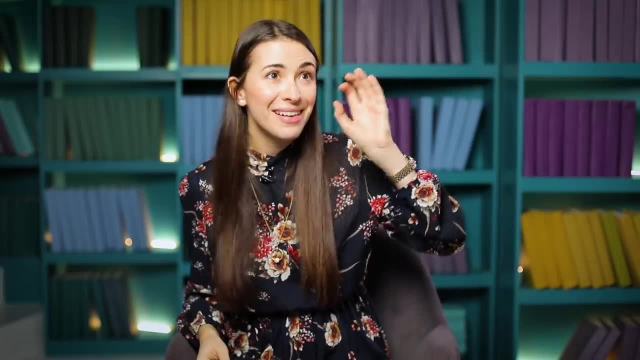 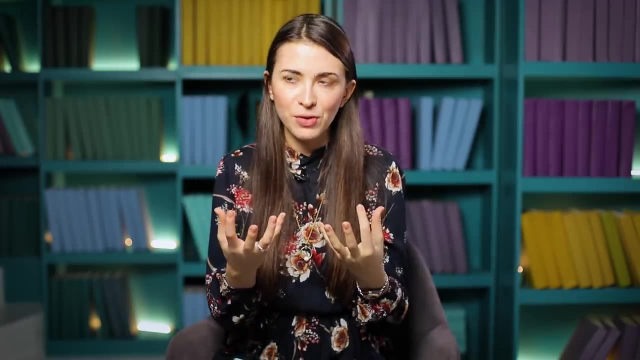 if you pronounce that, that's even better, because sometimes when we're thinking about something in our head, we just you know if we forgot the word, we just skip it. but if you're trying to pronounce it you're like: oh my god, i forgot this word. i need to look it up. 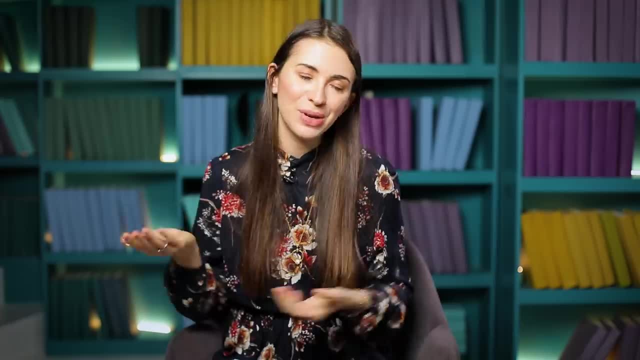 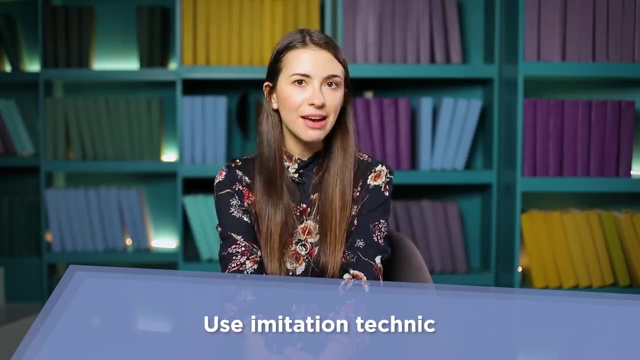 so pronounce everything where you're thinking. when you're home alone, it's a lot easier. the next tip i want to share with you is how to wait for your teachers for a semester right now. The next technique is called imitation technique. When you watch something on TV, you watch something. on Netflix, you watch something. 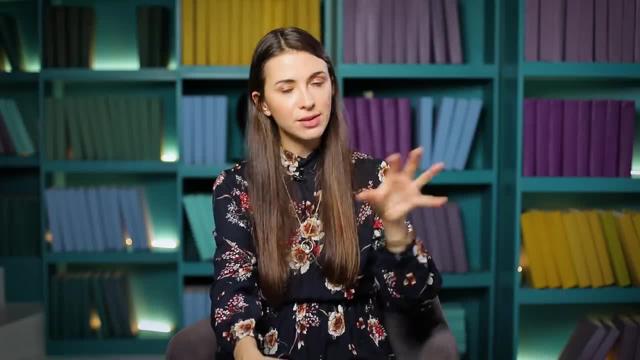 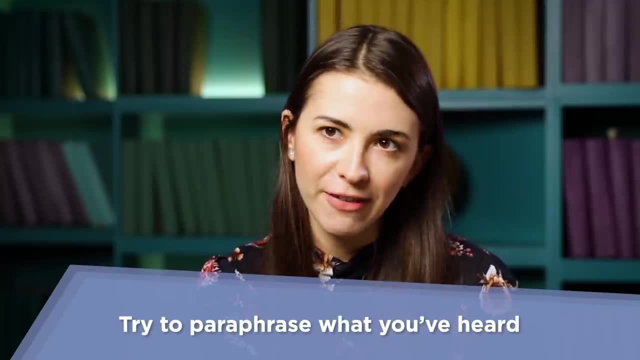 with subtitles. on YouTube, you can hear a phrase. read it, then pause, and not only try to repeat this phrase with the same intonation, try to paraphrase it, try to use some different words, because in this way, you would be sure that you understood the phrase and you would 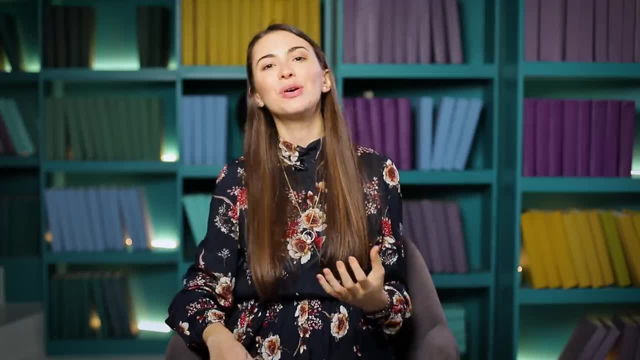 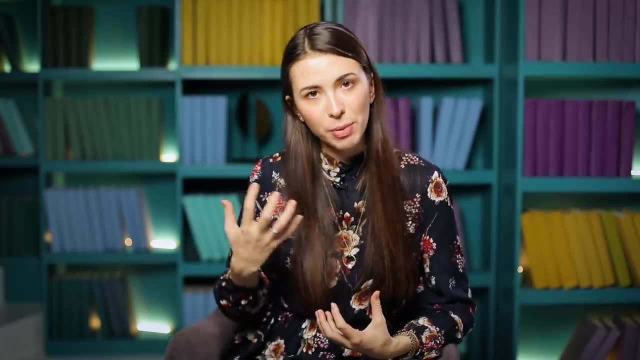 be practicing other vocabulary as well. So when you pause the movie or when you pause a video, just imagine that you're the character and try to pronounce that phrase in the same manner, replacing some words. I also suggest that you exaggerate whenever you're mimicking someone, because it's always 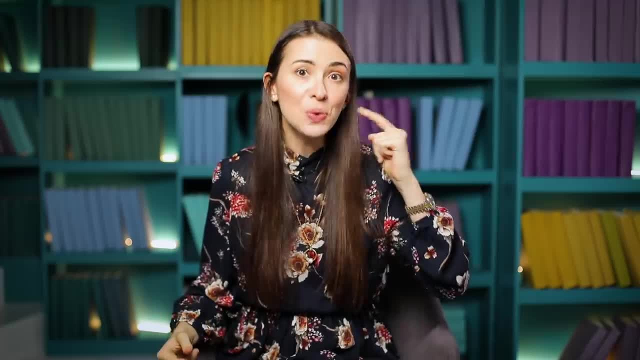 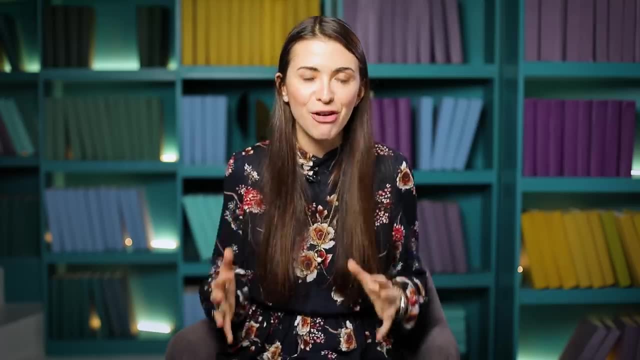 like that with the language. If you want to sound more natural, you would sound like you're being a clown to your brain and you would sound like you're exaggerating a lot to your brain. And that's the right thing to do, because when you are practicing a foreign accent, 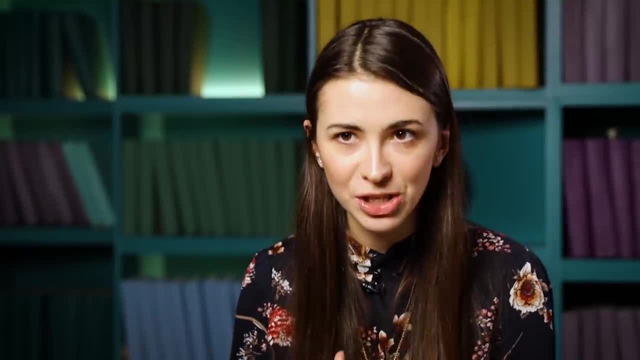 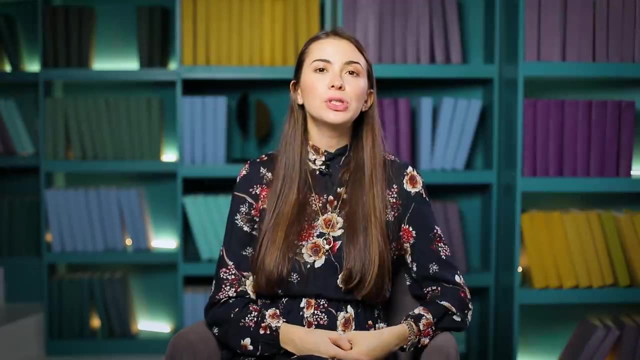 it would sound foreign to your brain, So try to exaggerate as much as you can Whenever you sound like a crazy person to yourself. that means that you're on the right track, And if you do everything that I mentioned in this video, your goal is to start thinking. 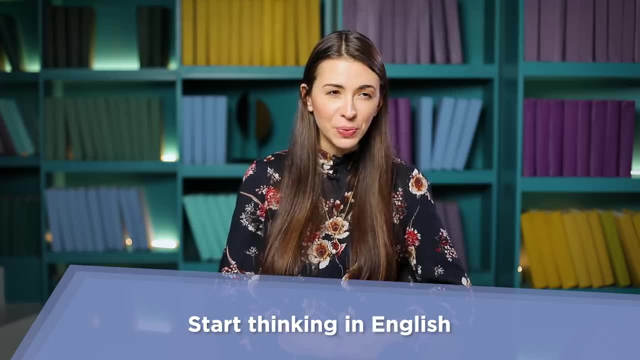 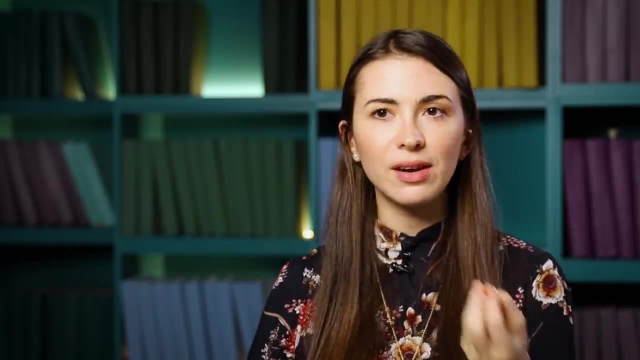 in English. That is a little hard. It's like meditation: When you meditate, people tell you that you have to stop thinking at all, And whenever you notice that you're thinking about something, you just notice that you're thinking about something and stop again. 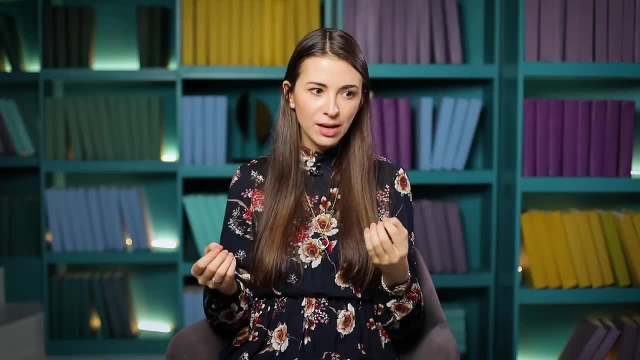 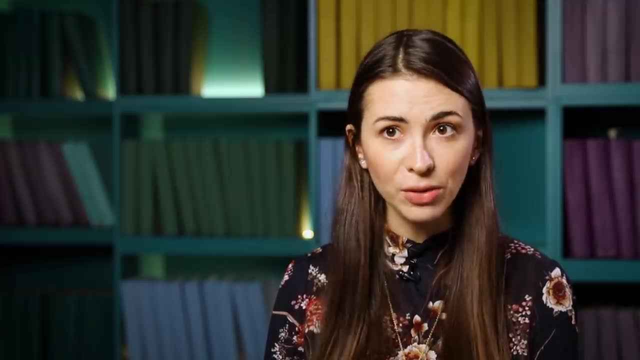 The same technique with thinking in English. You think in English and then you realize you're actually thinking in your own language. You don't punish yourself. You tell yourself: okay, I was actually thinking in my own language, so I just stop here and